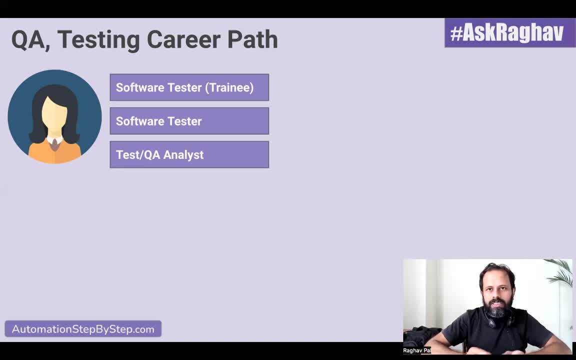 you will be involved in the testing and the QA process right from the beginning, where we discuss the requirements, where we discuss what should be the testing strategies, what should be the test plan, how we will manage the testing process, what user stories should go in, how we will test these user stories, what should be the tools involved, what should 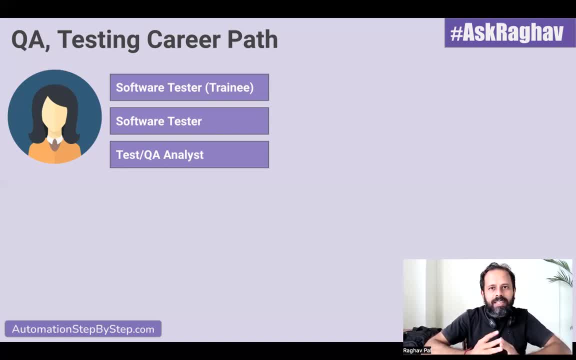 be the techniques involved, So you will have visibility in the complete QA process- the complete QA process right from the beginning till the end. You can then turn into a test or QA engineer. Now QA analyst or QA engineer, you will be doing more or less the same things as an engineer. in some organizations, We call this role as: 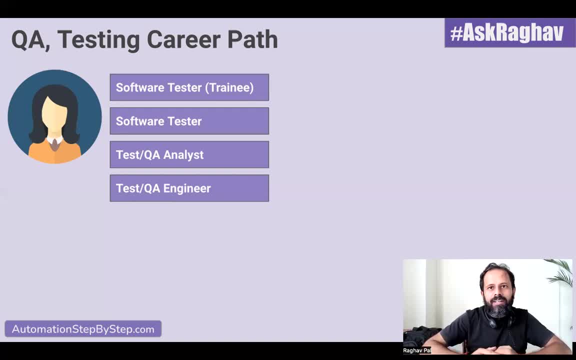 QA engineer, where you are more into the engineering side on, of creating the frameworks, solutions for testing process. So you will be doing all these things as a QA analyst and QA engineer. Now, until here, this is the technical part Here, most of the things you will be doing. 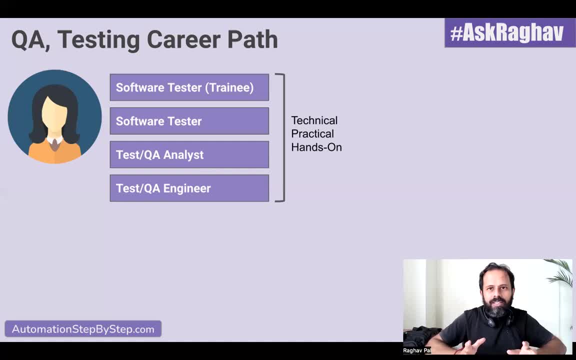 will be the practical hands-on And now from here. there are two parts. One is if you want to continue in the technical field and you want to be hands-on, or if you want to go into the management line Now from here. if you want to continue as a technical person, you can become a technical lead Now. 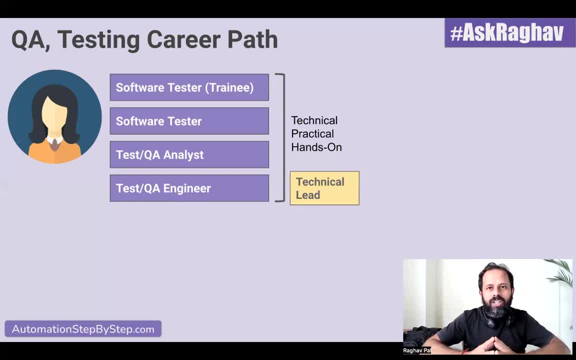 technical lead will be responsible for managing the QA testing team and he will be having more visibility in the tools used. the scripting part, The framework part and all the technical things are related with the QA and testing process. along with that Technical team management, Then you can grow into our test or automation. 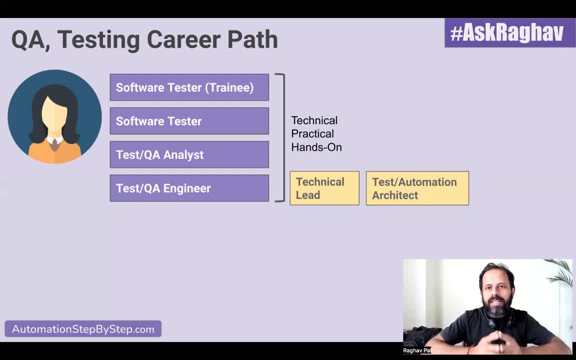 architect and here you will be Responsible for designing and developing frameworks, helping that in guiding the team in all the technical aspects. So you can convert into a test or automation architect And from here you can grow into an expert. for because until this stage you will be A lot of experience, A lot of QA engineers, A lot of skill setters. 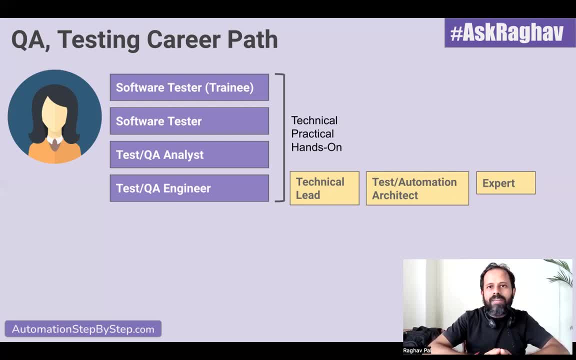 So now, what you are really talking about now is the overall N persecution of automation. That's something you can do. if you want to figure out how to improve, Then you can further set and then you can decide if you want to take some particular field and you can grow into an. 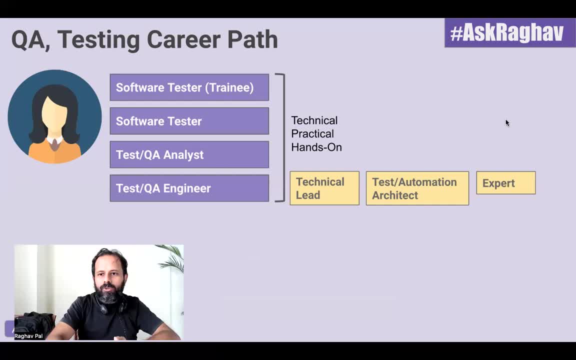 expert and here the different fields you can go into is: you can become an expert in the qa process, in the qa automation process, with different tools and platforms and skills required. you can grow into devops, engineer a devops person, and you can learn the different devops tools and techniques. 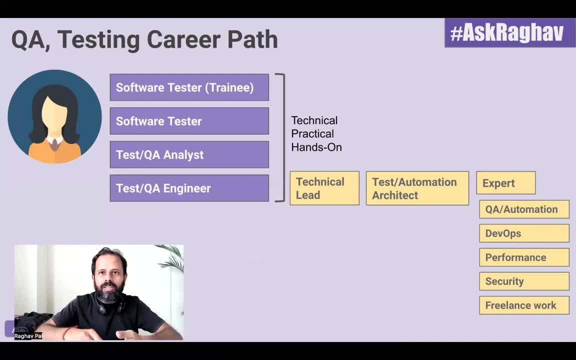 and platforms. performance testing is another very great field. you can become expert in performance testing or security testing. is there, then, after this? because until here you will have lots of skills, lots of experience. you can decide to continue in a job or you can also do freelancing. 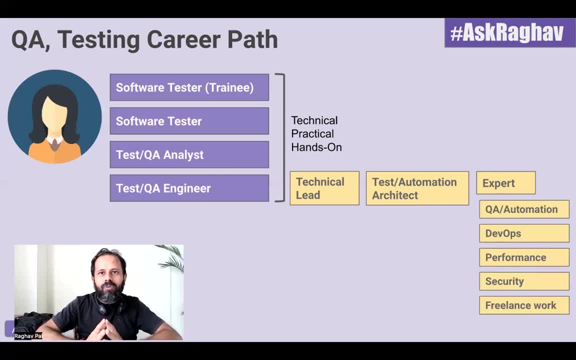 now here. if you decide and if you want to become a freelancer, always first start along with your job and then see how you are performing- can you do it full-time or not- and only after that you can decide to decide to become a full-time freelance person. 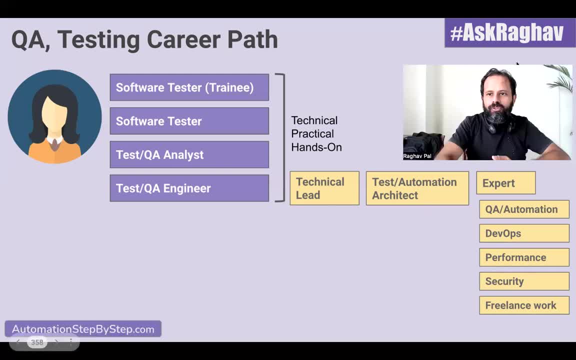 now, this was the technical field. if you want to continue in the management line after test or qa engineer, you can become a test or qa lead and here you will have more uh work as management, management of team, management of people and resources, and less technical hands-on work. 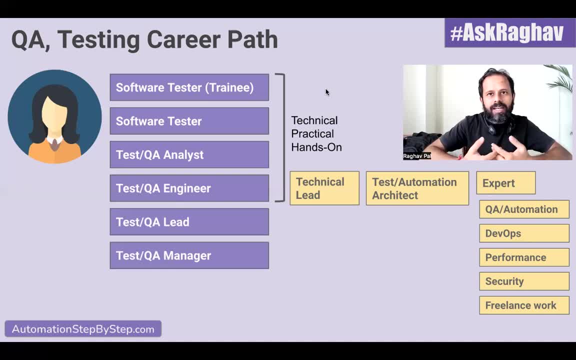 then you can grow into a test or qa manager. again it will be more people and management things here and then you can go into the senior management roles in the organization or in the qa process. so this is less technical and more management and more people skills here. so you can decide. 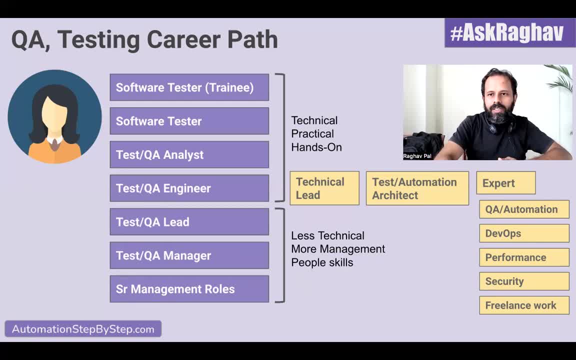 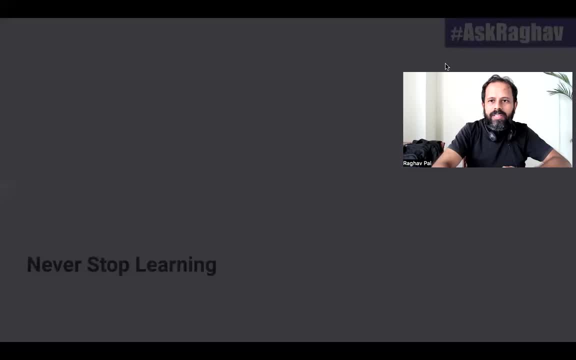 which uh path you want to grow into in the testing and qa process. so this is the complete career path. if you want, you can take a screenshot of this screen and keep it handy with you and with that uh, we will stop this session here. if you have any more questions for me for the 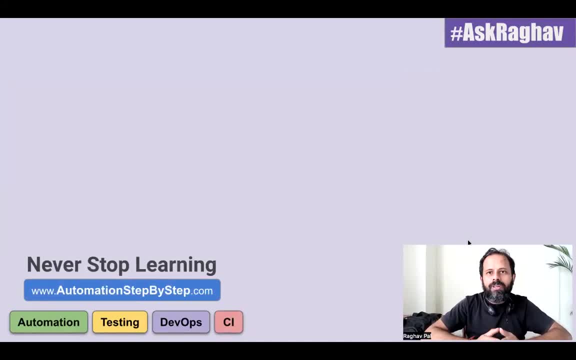 next episode of ask raghav? you can let me know in the comment section below you. i will see you soon. thank you for watching and never stop learning.